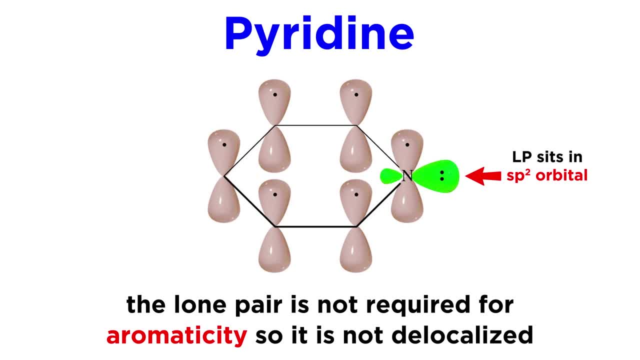 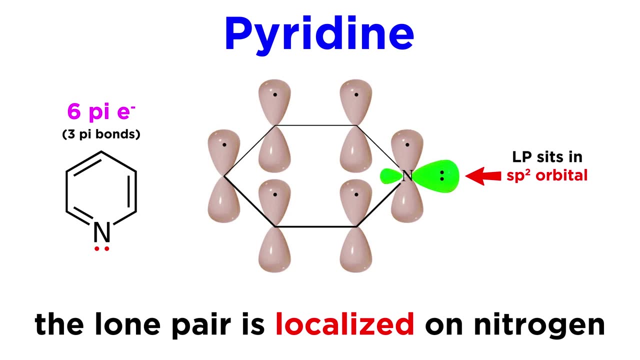 does not delocalize, as it is not required to participate in resonance in order for the molecule to be aromatic, The six pi electrons from the three pi bonds are sufficient, so this lone pair is actually localized on the nitrogen atom. For this reason, pyridine is much more basic. 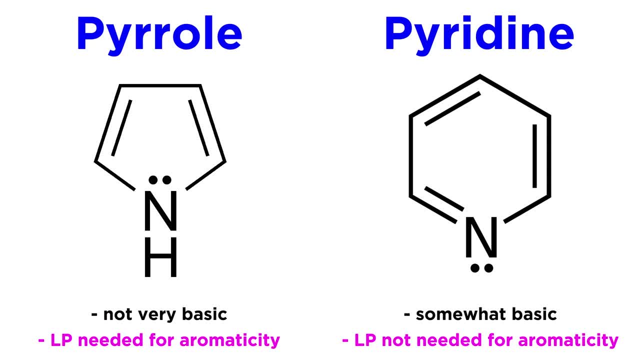 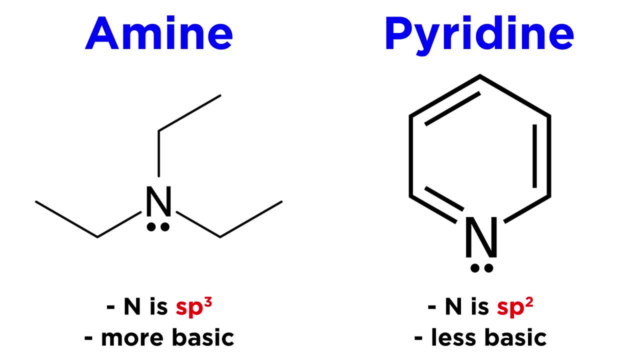 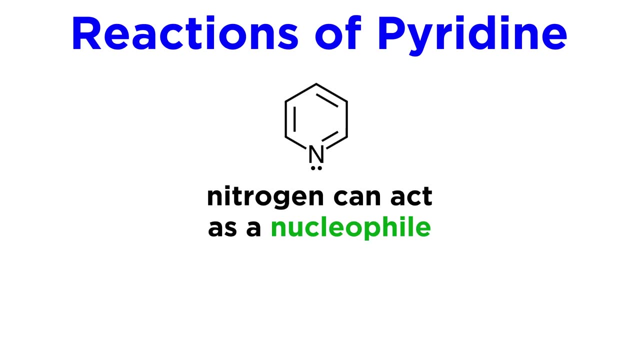 than pyrrole, as the lone pair is available to act as a proton acceptor, though not as basic as a regular amine, given that sp2 orbitals have more s-character than sp3 orbitals, meaning they are held a little closer to the nucleus. In addition to acid-base chemistry, pyridine, 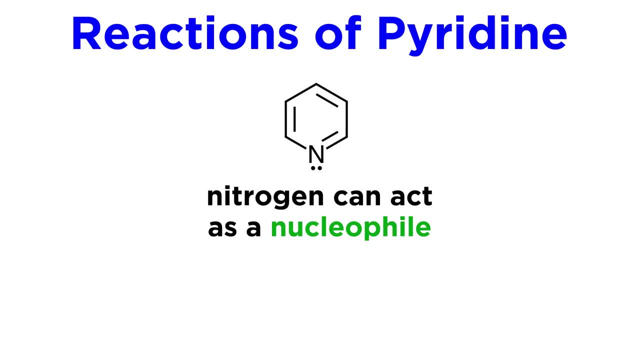 reacts similarly to other amines. as an n-based nucleophile, It can undergo alkylation with an alkyl halide or acylation with an acyl chloride, yielding a highly reactive N-acetyl pyridinium salt. Oxidation with peroxy acids is also possible. 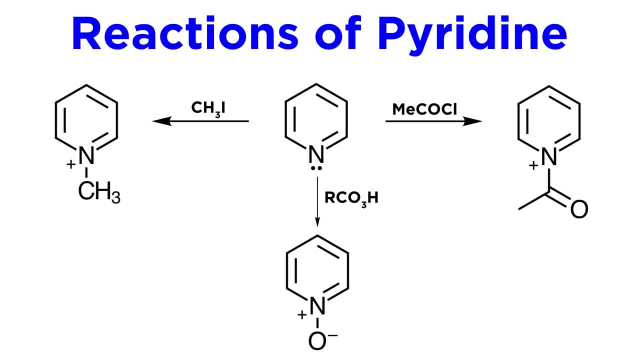 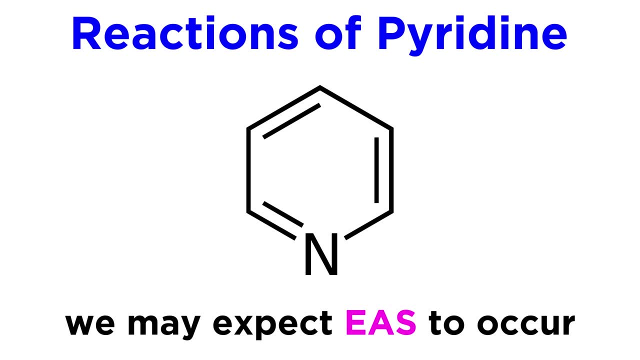 yielding a stable pyridine oxide. Now, as an aromatic system, we might expect pyridine to undergo electrophilic aromatic substitution, like benzene derivatives and electron-rich heteroaromatic systems such as those in the previous tutorial. However, this is not the 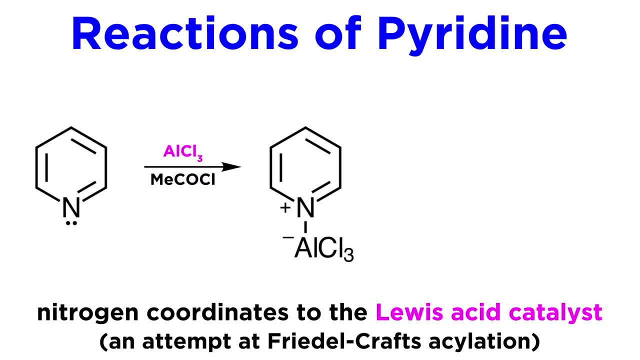 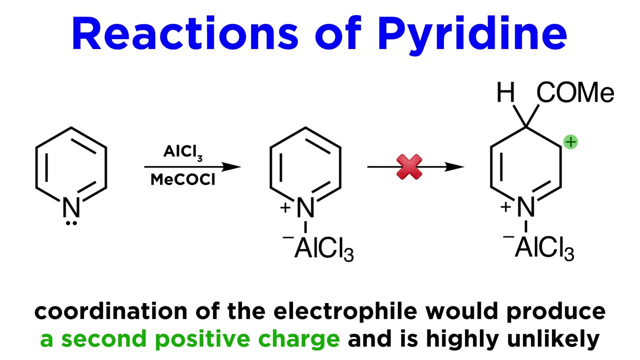 case due to the N effect. Whichever lewis acid would catalyze the relevant substitution, the nitrogen on pyridine will coordinate to it, being nucleophilic, And this renders electrophilic attack highly unlikely, given that it would result in yet a second formal. 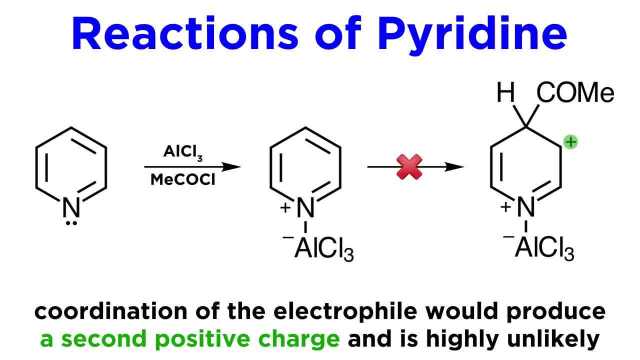 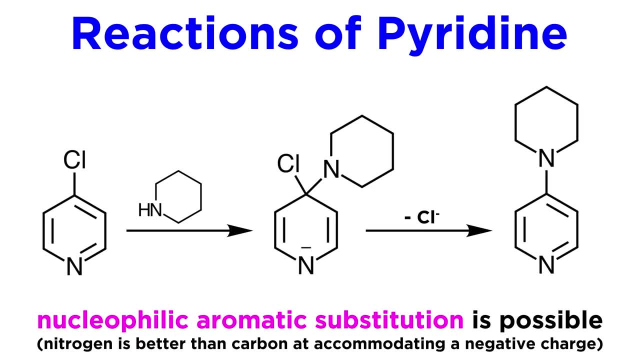 positive charge, such as here, if Friedel-Craft's acylation were to occur. so this is not a likely process for pyridine. However, nucleophilic aromatic substitution is feasible, given nitrogen's greater ability to stabilize negative charges over carbon. This can therefore occur without any kind of activation needed. 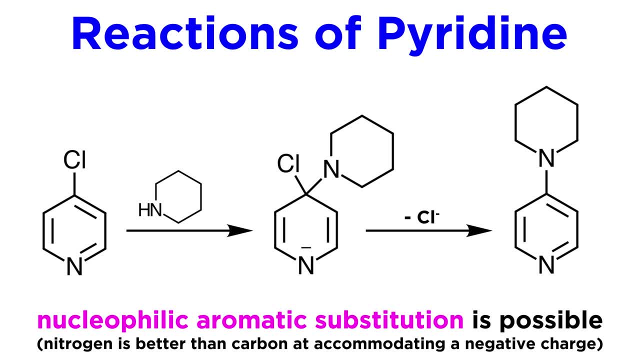 such as with the reaction below. The mechanism for this type of reaction was discussed in another tutorial, but to review, in this case, piperidine attacks the electron-deficient carbon bound to chlorine, which pushes a negative charge onto nitrogen. This can then come back up to kick. 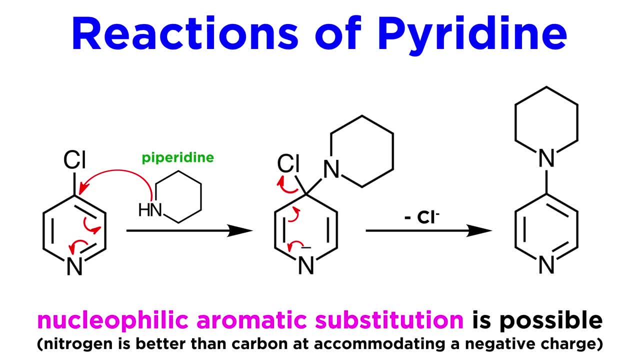 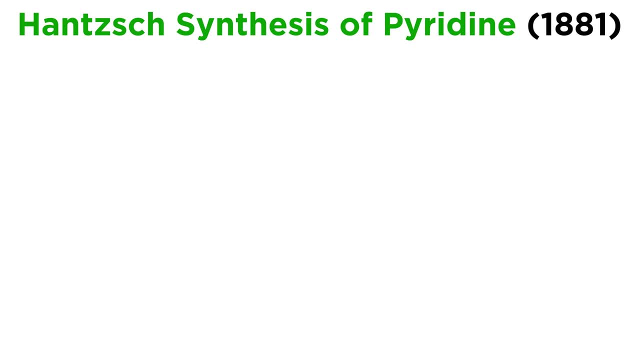 off the chloride ion, generating the following product: In terms of pyridine synthesis, the most widely used method is the Hantsch synthesis, developed by German chemist Arthur Rudolf Hantsch in 1881.. This has four components: two beta-keto- 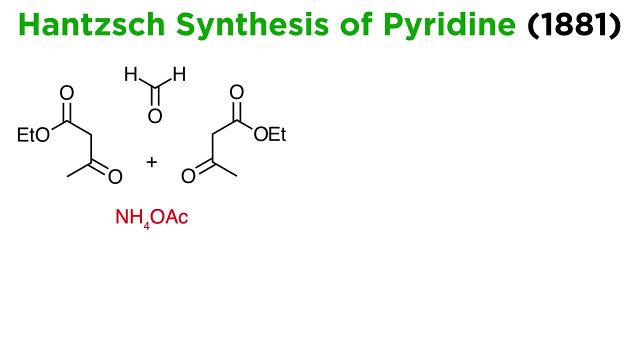 esters: formaldehyde and ammonium acetate. Under aqueous conditions, this yields a dihydropyridine which is then readily accessible to the human body. This is also known as dihydropyridine, which is also known as dioxidized. to produce the aromatic system, A variety of esters can be used. 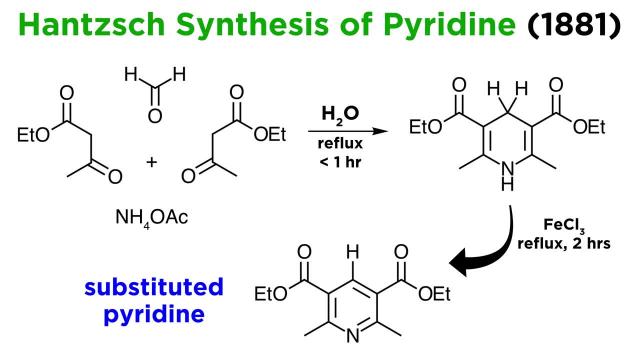 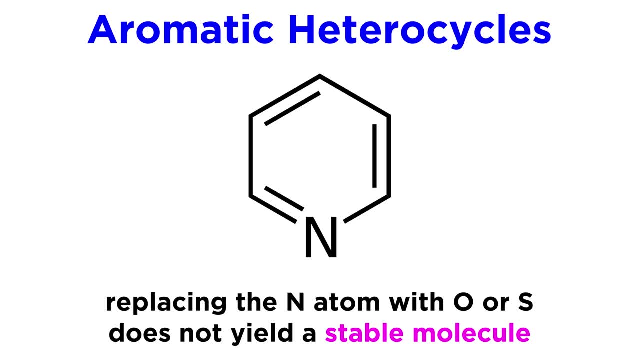 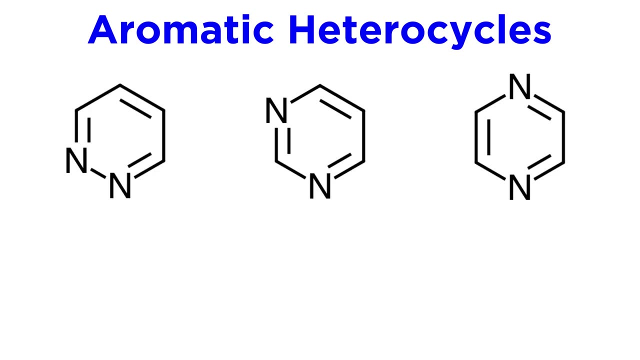 to produce non-symmetrical pyridines as well. Unlike the five-membered heterocycles we've examined with six-membered rings, replacing nitrogen with oxygen or sulfur does not result in a stable, neutral species, so these will not be discussed. However, there are stable derivatives. 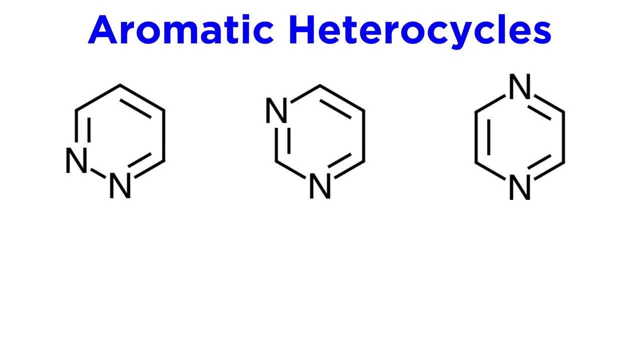 of pyridine that have two nitrogen atoms instead of one. There are three such structurally numeric structures. If the two nitrogens are adjacent, we get pyridazine. If two apart, it's pyrimidine, and on opposite sides it's pyrazine. These are all weaker bases. 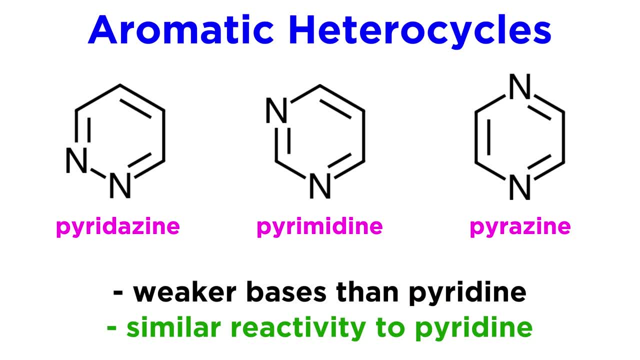 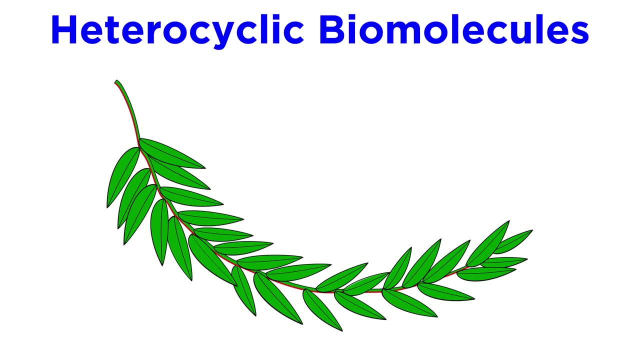 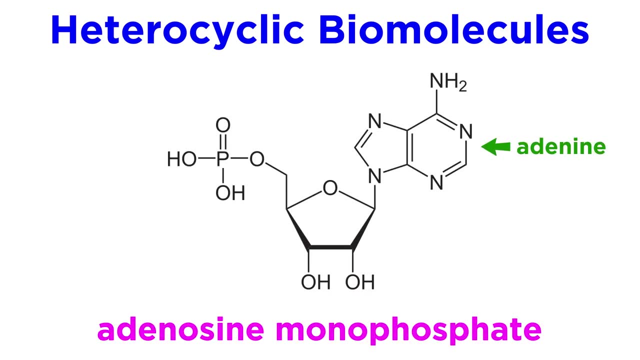 than pyridine, although they share similar reactivities. Heterocycles of this variety are omnipresent in natural products, so it is clear that nature has devised an efficient route towards producing these biological subunits. For example. we need look no further than to produce a subunit of pyridine, For example. we need look no. 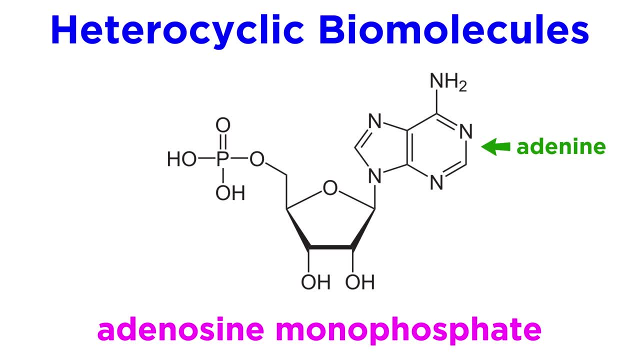 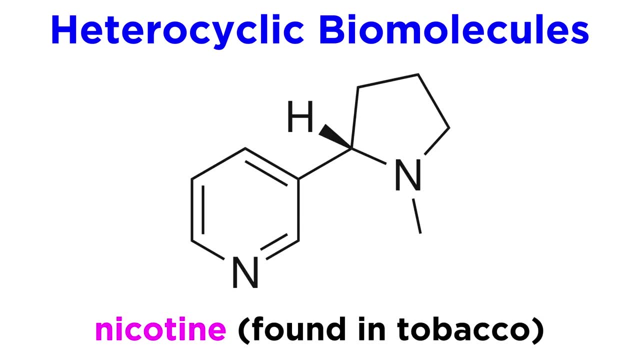 further than to produce a subunit of pyridine, For example. we need look no further than the nitrogenous bases in DNA such as adenine. There is pyridoxine, also known as vitamin B6.. Most of us have heard of nicotine, the addictive component of tobacco, And then there is quinine. 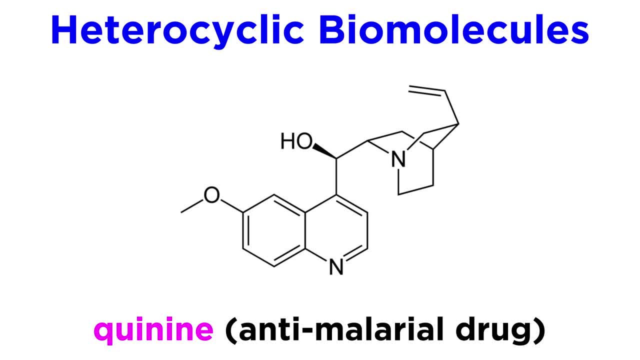 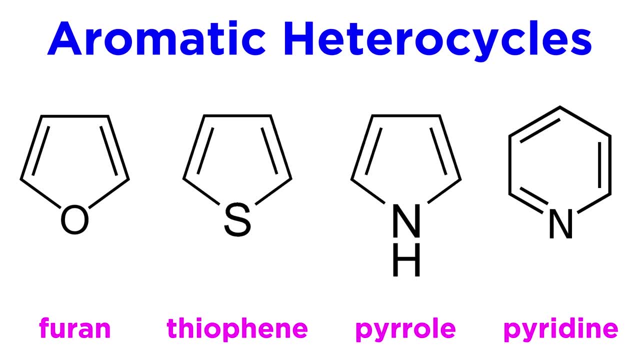 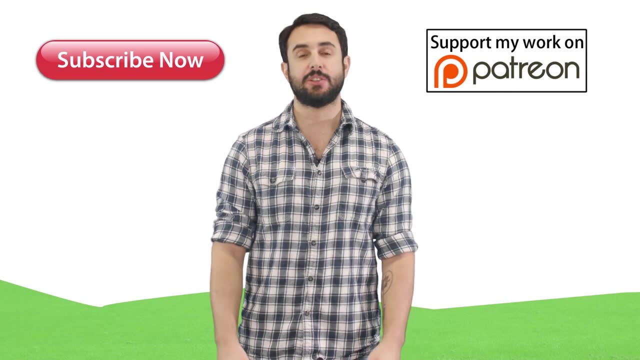 an anti-malarial drug. that was the focus of one of the tutorials in our study of the history of drugs, And with that we have a preliminary understanding of some important heterocycles. Subscribe to my channel for more tutorials. support me on patreon so I can keep making. 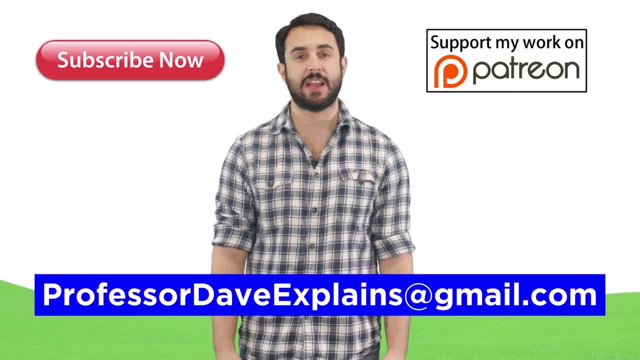 content and, as always, feel free to email me professordaveexplains at gmail dot com.